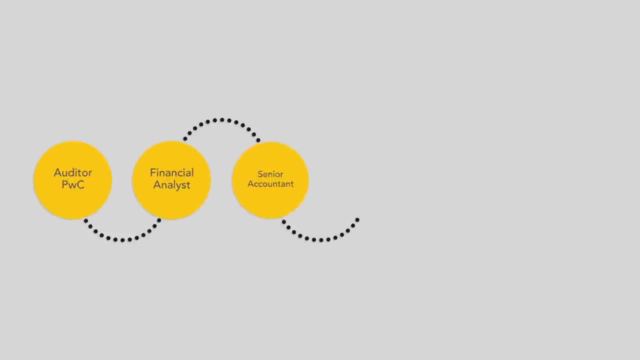 field of finance, Where I started out at PricewaterhouseCoopers as an auditor and then I transitioned out to private industry and then I worked my way up from a financial analyst position all the way up to a corporate controller position, which is what I do today, And this channel is all. 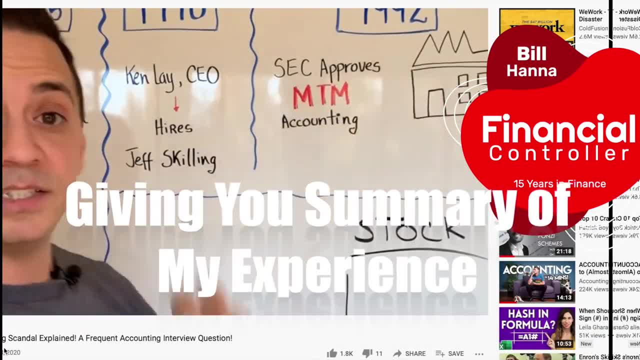 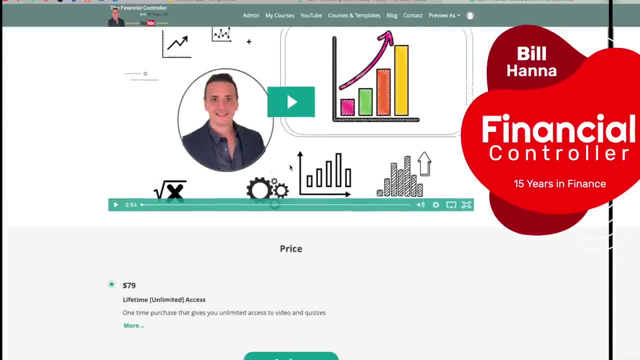 about giving you the summary or the juice of my experience over the last decade and a half, And I do this here in the YouTube channel as well as on my website through blog posts and online course and templates, So go ahead and check it out. 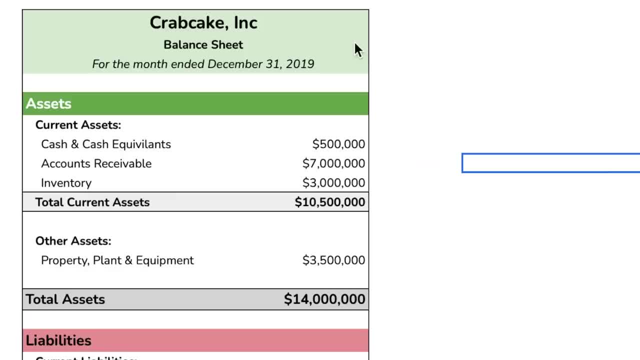 Check that out as well. All right, So diving into the balance sheet here. This is a balance sheet for a company called Crab Cake Inc. and it's for the month ended December 31, 2019.. And, as we all know, the balance sheet shows the financial position of the company at a point in time. 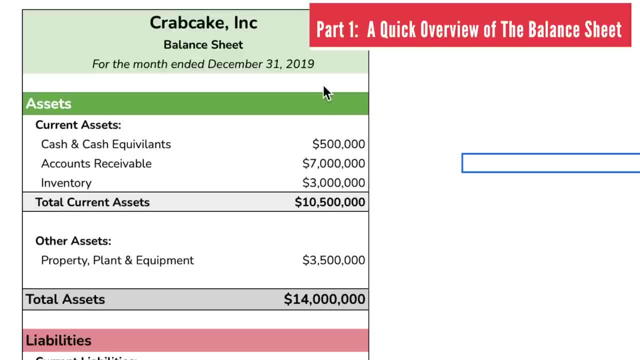 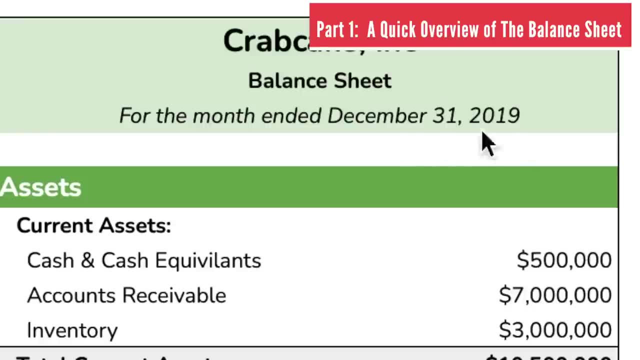 This is as opposed to the income statement, which shows the financial performance of the company during a period of time. So here we're looking at a point in time which is December 31 or December 31st 2019.. And the basic structure of the balance sheet is as follows. 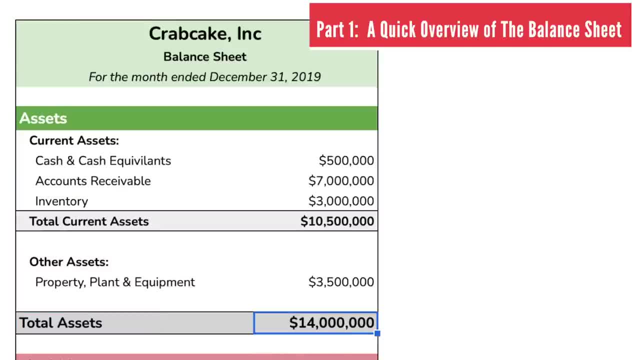 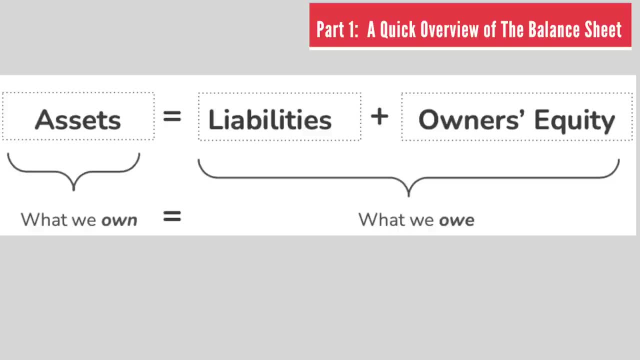 It shows that total assets, which is 40 million in this case, will always equal total liabilities and equity, which is saying that assets equals liabilities plus owner's equity. Assets is what you owe equals what you own. So obviously, assets is what you own in the company will always equal what 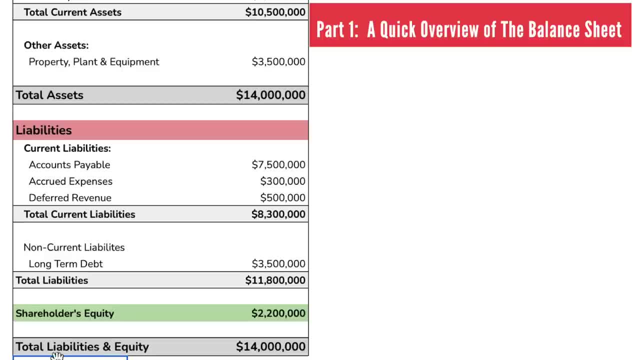 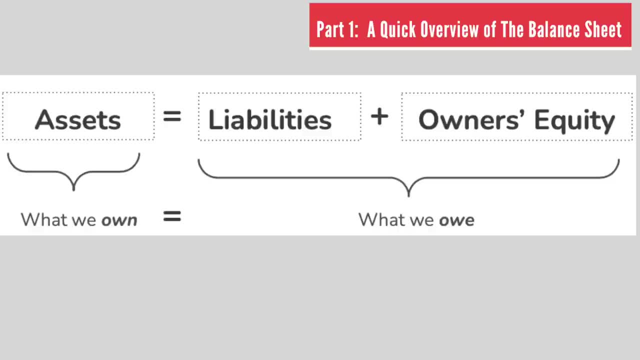 you owe, which is total liabilities and equities. Obviously, liabilities is something that you owe to third parties and equity is also something that the company owns, but it owes to the owners of the company, Right? So it's very easy: What you own in the company or assets will always equal what you owe, which is: 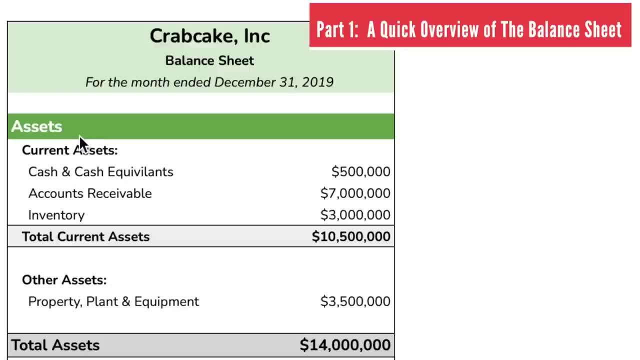 liabilities and owner's equity. All right, so let's go over assets real quick. So for assets, we'll always have current assets and then non-current assets or other assets. So basically, current assets are those assets that can be converted into cash within 12 months. So when we look at current assets, it will include cash or cash. 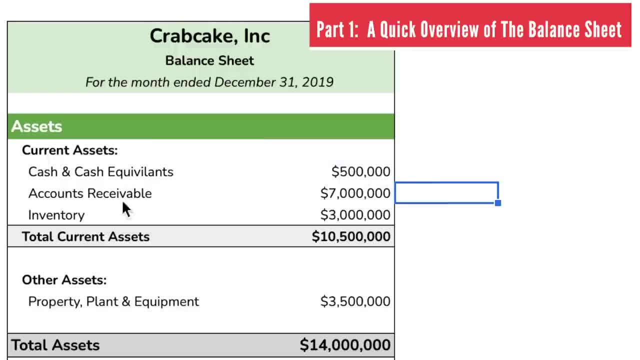 equivalent. Here we have half a million dollars, We have accounts receivable, which is always. the assumption is that you can turn it into cash within 12 months because you'll collect your accounts receivable, And then inventory, which is $3 million in this case, And the idea is that all of these components, all of these three items on. 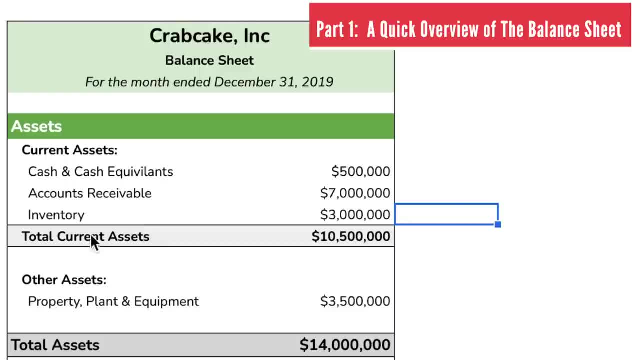 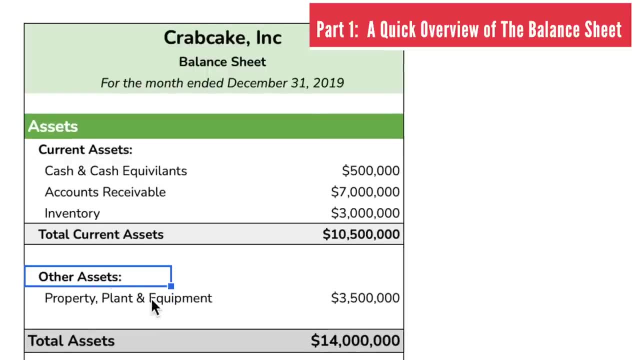 current assets can be converted into cash within 12 months, And that's why we call it current Right. So current means that it can be converted to cash within 12 months. And then we'll always have the other assets, or non-current assets, which is, in this case, property, plant and equipment, because the idea is 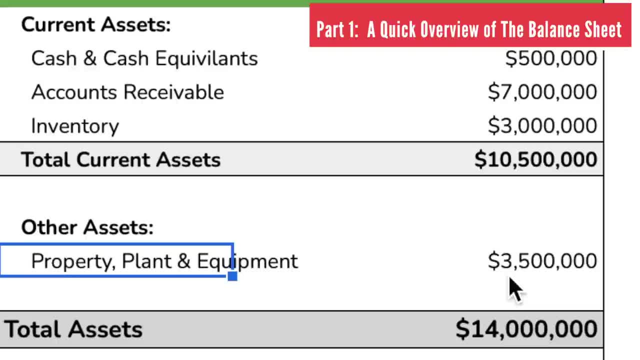 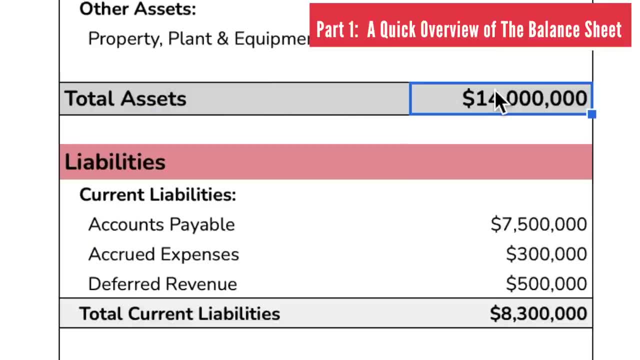 that these are an investment in the future of the company. This is not something that the company owns. It's something that the company intends to sell and turn into cash, And so this is other assets here. So the total assets for the company is $14 million, And then we can jump over to the liability section. 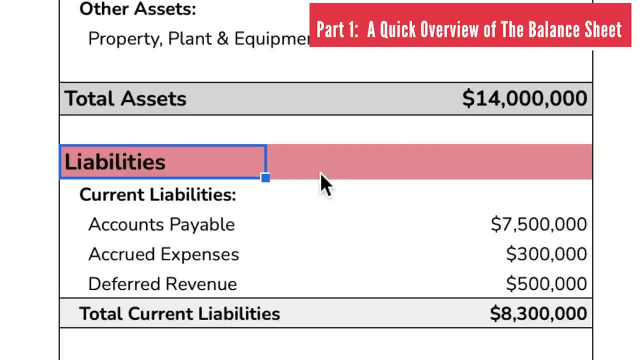 So liabilities are also broken down in a similar fashion to assets, where we look at current liabilities And then we look at non-current liabilities. So current liabilities- similar concept- These are the liabilities or the obligations that are expected to be fulfilled, that the company has to fulfill within 12 months. 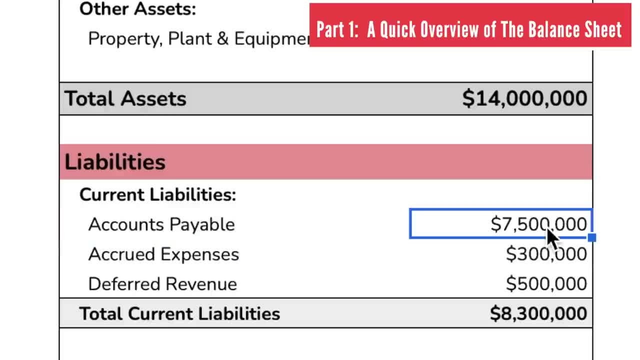 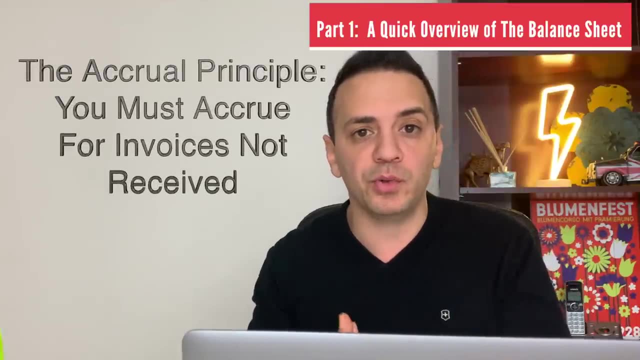 And so an example here is: accounts payable pay its accounts payable within 12 months, of course, and then you have accrued expenses, and these are the all of the other expenses that the company hasn't yet booked as payable. but based on the accounting principle, of the accrual principle, the company needs to accrue for any liability or 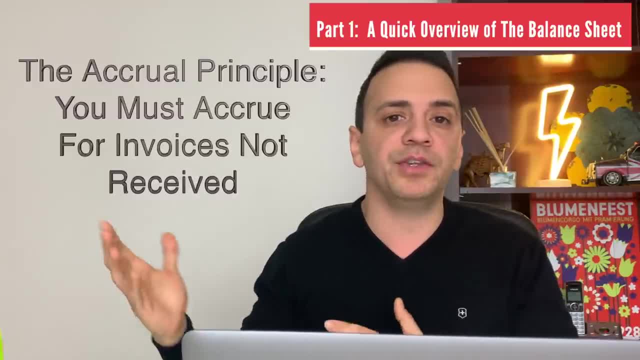 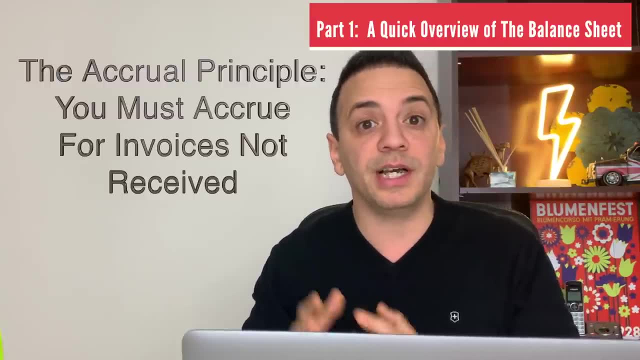 obligation that it hasn't received an invoice for. so, even though you haven't received received an invoice for a service or a product from a vendor, you still need to accrue for it, and this is based on the accrual principle right. this is one of the principles of accounting: the accrual principle. 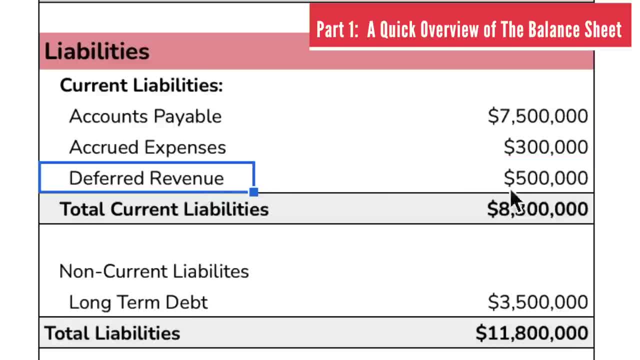 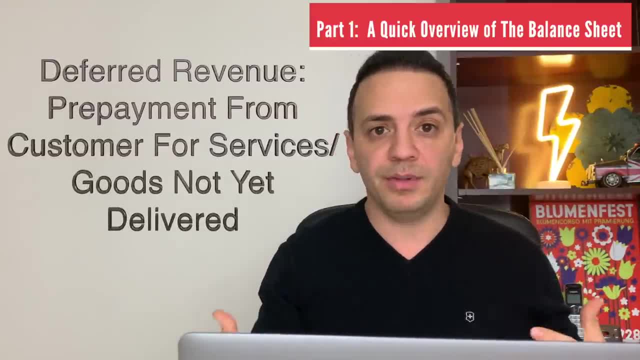 so accrued expenses- 300 000, and then we have deferred revenue- 500 000. the first revenue basically is you can think of it as pre-payments from customers. so as a company, you're receiving cash from your customers for a future product or service that you will deliver to them in the 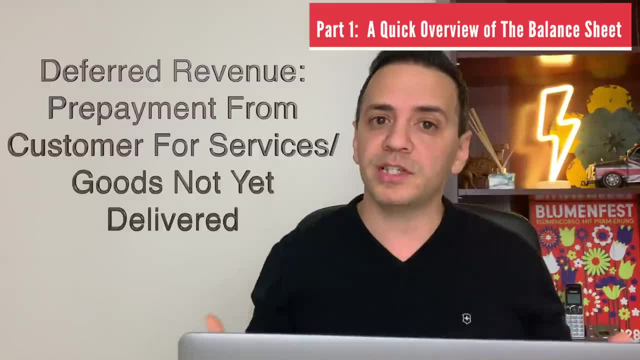 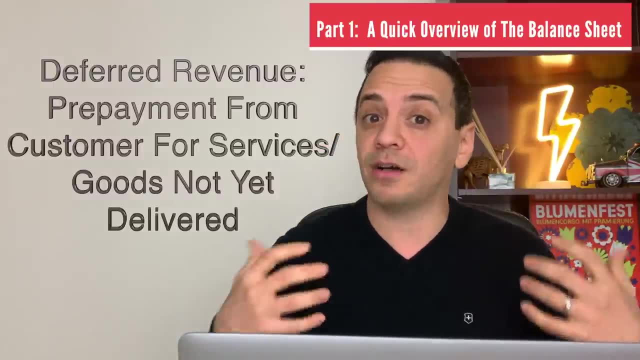 future. but the reason why we record it as a liability is because this becomes an obligation for the company, right? so you receive cash, you record the cash as a debit, but then your credit is deferred revenue, which is a current liability, because this is still an obligation for the 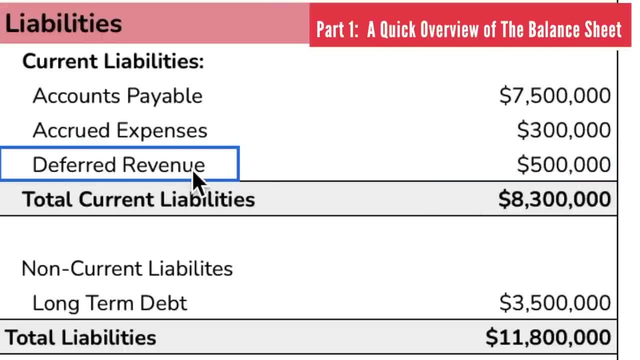 company to fulfill, and so 500 000 in this case is deferred revenue, and that will give us a total current liabilities of 8.3 million dollars. and then we'll jump over to non-current liabilities, and these are the liabilities that we don't expect to pay for the next 12 months. so here we have a long-term loan. 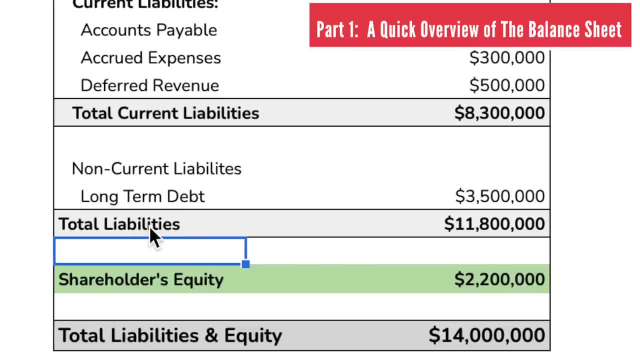 or long-term debt of 3.5 million dollars, and that gives us total liabilities of 11.8 million, and then, after that, what's left over is going to be the stockholders or the shareholders equity of 2.2 million, which can be- you can think of it as subtracting total. 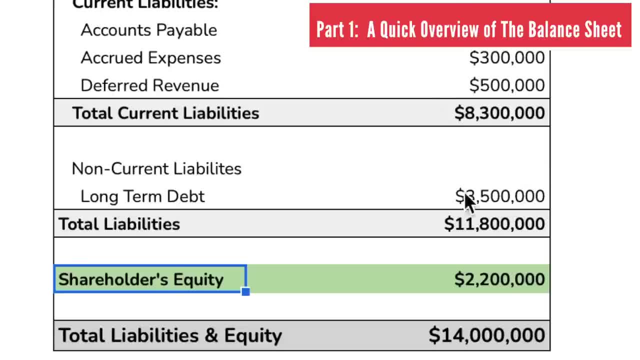 liabilities from assets. so if you take all of the liabilities and pay it off from the assets, what's going to be lifted over here is 2.2 million dollars, and this is the what the owners of the company can claim as their equity in the company: 2.2 million dollars. 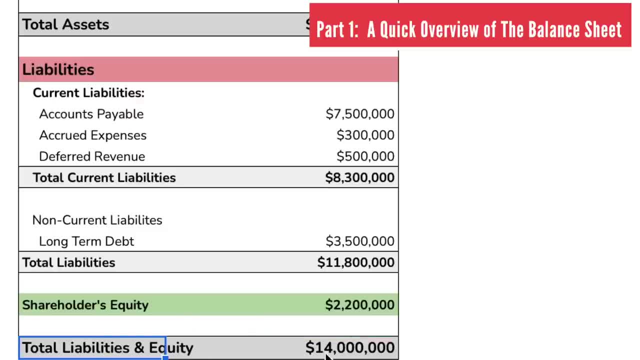 in this case, and then, obviously, as we said, total liabilities and equities. 14 million dollars is going to always equal total assets, or 14 million, and this is one of the first things you look for when you're analyzing a balance sheet right. is total assets equal to total love ability? and 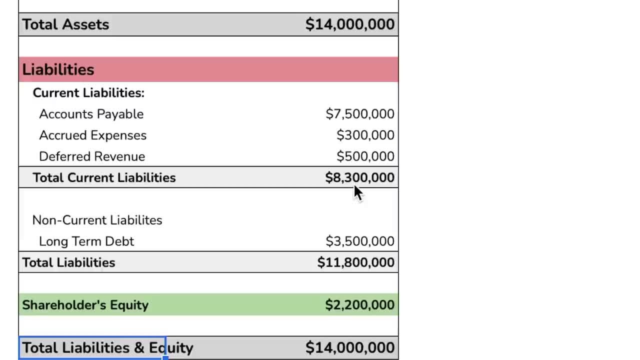 if they're not equal, then you're looking at a balance sheet that has an error in it and you need to have that error looked at first before you can even begin to analyze the balance sheet. so the first thing is this number: here assets need to equal total liabilities and equities. 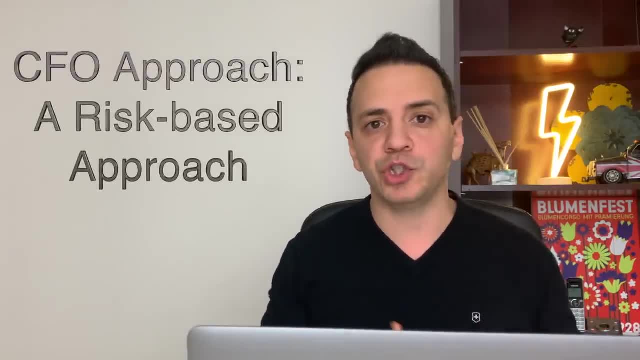 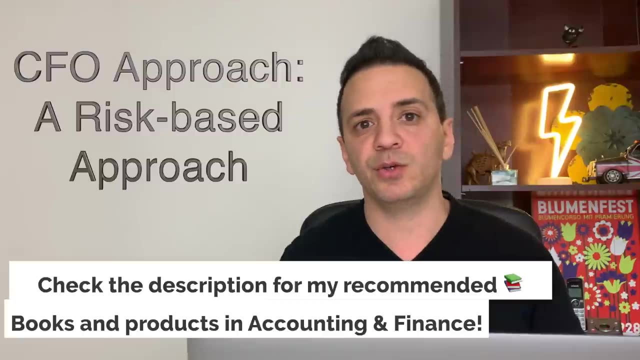 and now that we've seen a quick overview of the balance sheet, let's talk about the approach of a cfo. how does the cfo approach the balance sheet? and we said at the beginning of the video that it's a risk-based approach, or what are the risks associated with each line item on the balance? 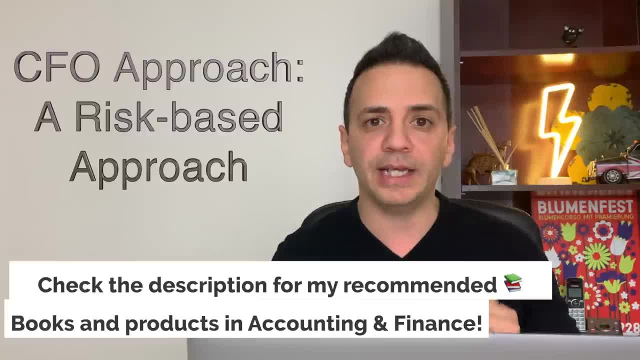 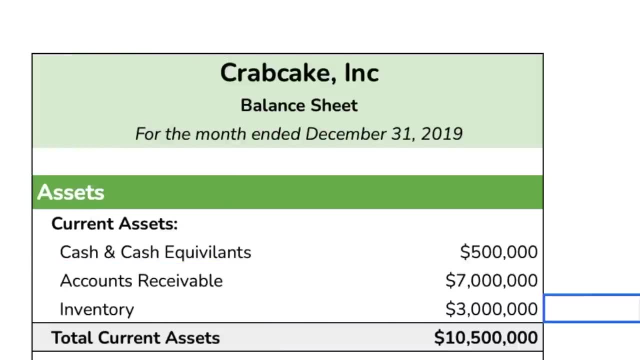 sheet. so let's dive right back in and look at the risk associated with each of the line items. uh, beginning from the assets and going down all the way to liabilities. all right, so starting with current assets, the first item here is going to be cash and cash equivalents, so a cfo will look at 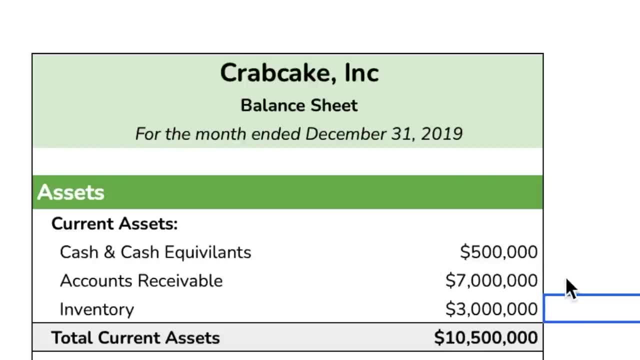 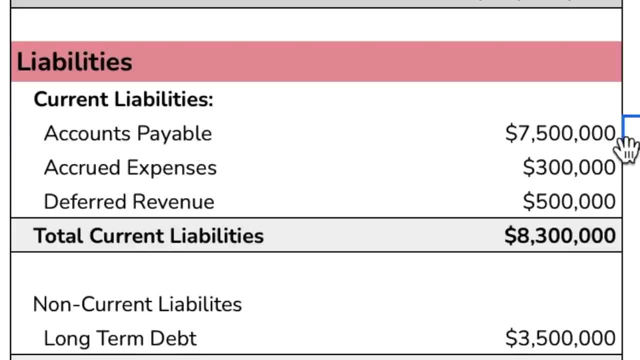 this number and say, okay, i have half a million dollars in cash. i need to look at my current liabilities. so look at accounts payable here and i'll see that my balance is 7.5 million dollars, which basically is telling me that i need to pay off the vendors 7.5 million dollars over the next. 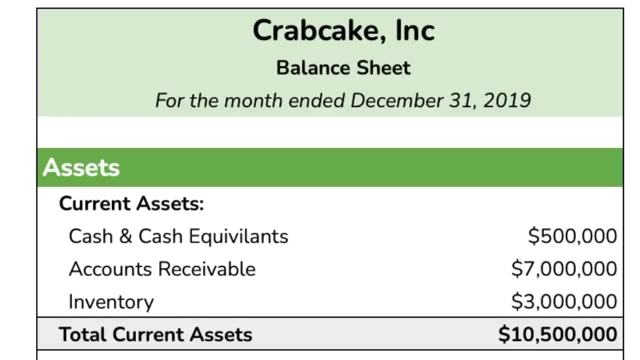 say 60 to 90 million dollars, so that's the first thing that i need to pay off the next 60 to 90 days. so i'll look here and say, okay, where is the money going to be coming from to cover all these accounts payable if i only have half a million dollars in cash? basically, i look here at accounts. 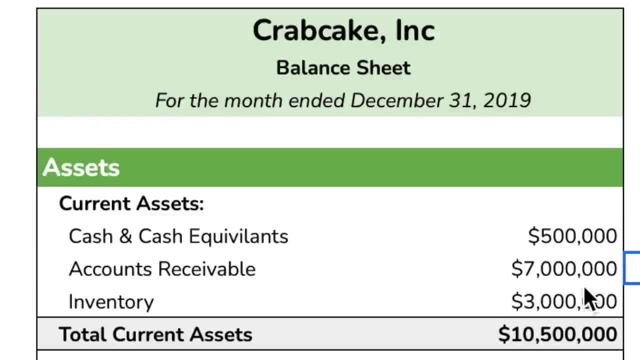 receivable and i see that i have a big balance, so seven million dollars in accounts receivable. this is expected to be collected normally in the course of business, uh say, between 45 to 60 days. so i'm expected to collect this number first, uh, so that i'm able to pay off my accounts payable. 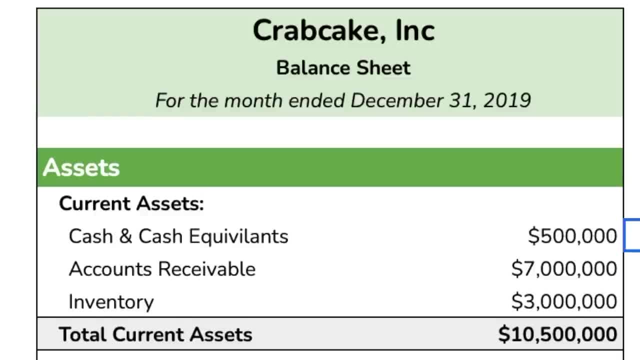 so this is the first thing that the cfo will look at, which is the obligations. so the cfo looks at the obligations of the company, uh, in relation to the cash position of the company to determine whether there's enough cash on hand to cover the obligations that are coming right up, and then the 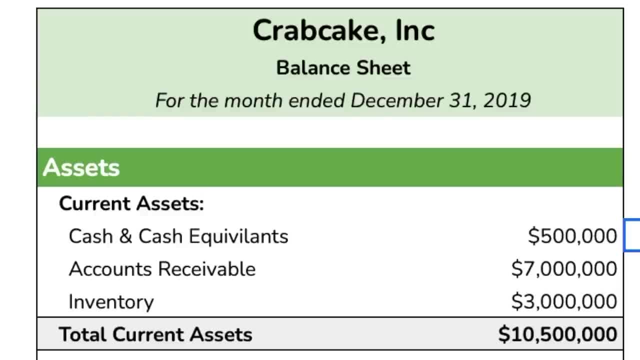 second thing that the cfo will look at is profitability. so we we know that the accounts receivable- seven million dollars- is going to cover um the obligations that the company needs to pay in the next, uh say, 90 days. but then what about profitability? is this company profitable? 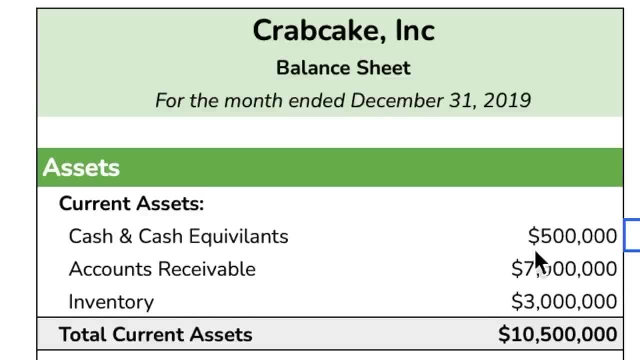 meaning? is this a cash machine? if my cash is running low here- and it's half a million dollars, am i making enough profits to be able to generate, to generate more cash, so that i'm hedging against the risk of running out of cash? so, basically, when we look, 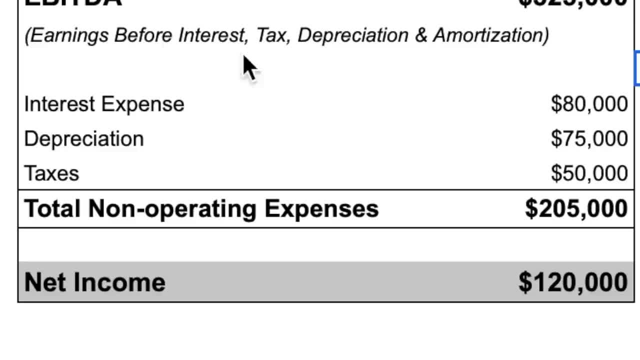 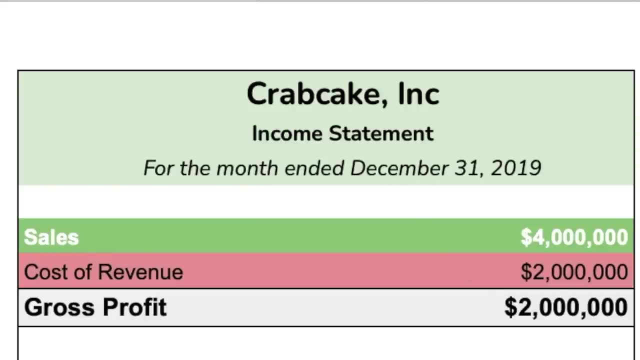 here at the income statement. uh, looking for the company's income statement and we see that net income is 120 000, which is adjusted for depreciation. when you put back depreciation, this is close to 200 000 for one month. so this is for the month of december 2019. so i can say okay on a. 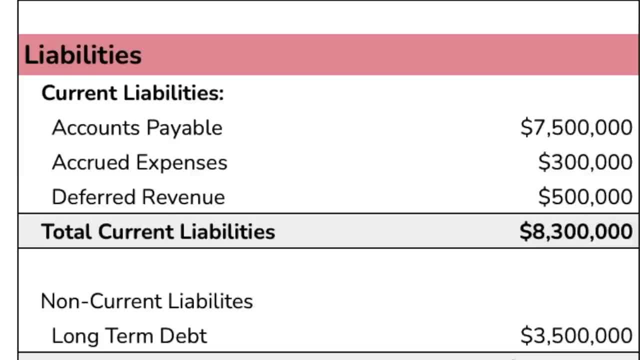 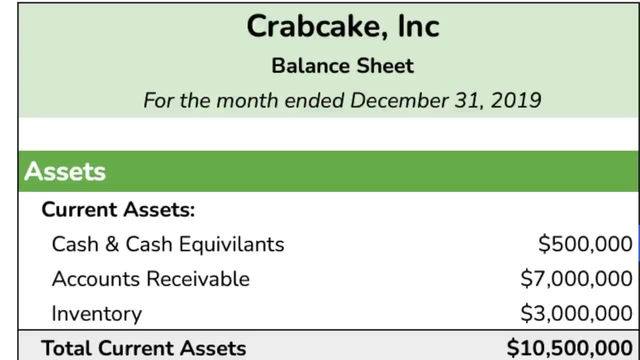 month of december 2019, i'm going to be profitable by about 200k uh, which gives me a little bit more comfort, uh that, um, over the course of a year, let's say, i'm going to be generating somewhere around two million dollars in profits, which will generate more cash to uh improve my cash position. so to 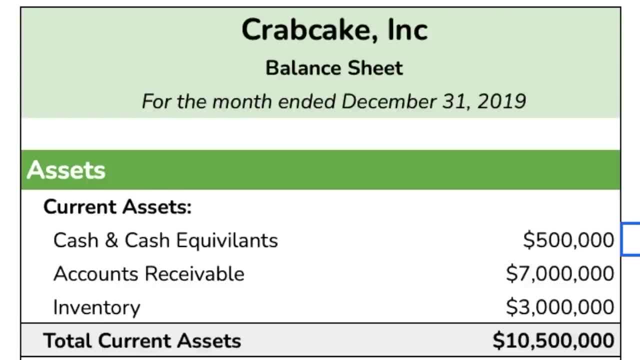 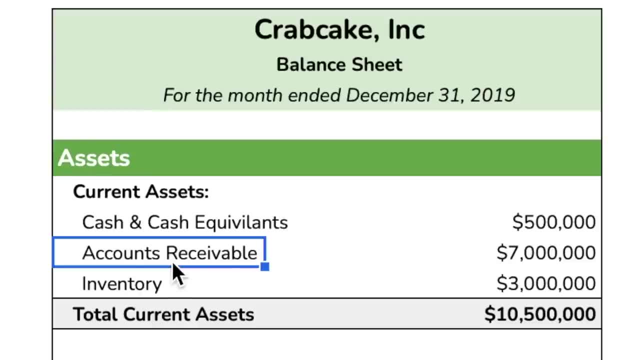 summarize: for the cash at cash equivalent, the cfo will be looking at uh, two things: obligations and then also looking at profitability, which in turn will create cash flow. the next item here in current assets is going to be accounts receivable. so the cfo would look at two things when it comes to accounts receivable. 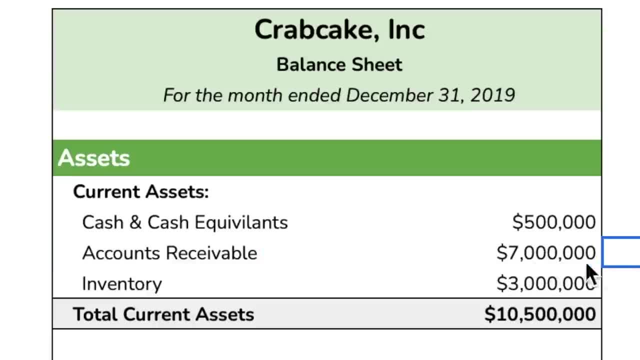 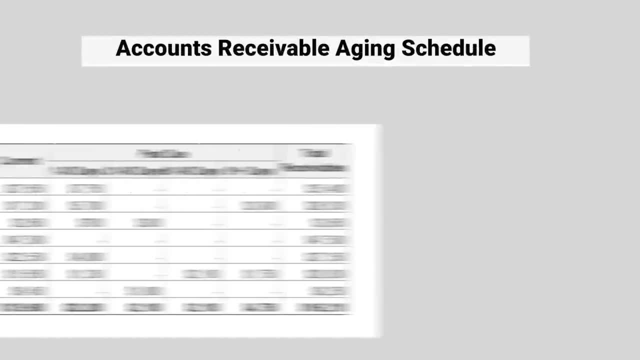 the balance and they'll say, all right, it's seven million dollars. so, uh, i need to see an aging schedule over the seven million dollars. so the aging schedule is going to show you the breakdown of this seven million dollars in terms of what the customer owe. uh, by buckets. so the first bucket is: 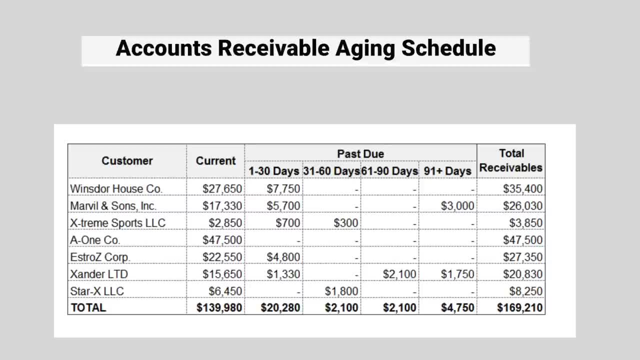 going to be current accounts receivable, or you know the accounts receivable that the customer is not late on paying yet, and then it's going to show you then the breakdown from 30 days, 60 days, 90 days, uh, so this way you can get an idea of like how much of this number is aged. 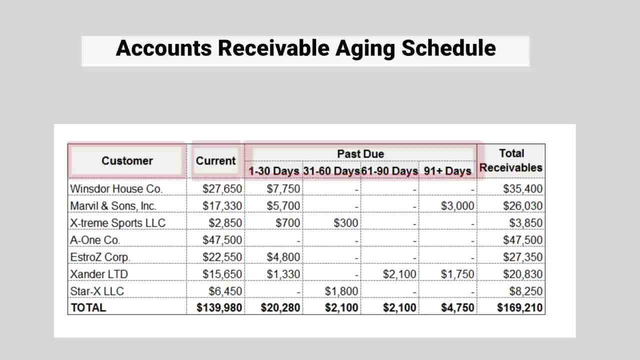 and that can give you an idea on how much of this number can be expected to be bad debt. basically, the customer is never going to pay this number, so the older the accounts receivable, the more likelihood that you're not going to collect it. so that's why it's important to look at that aging schedule of accounts receivable. 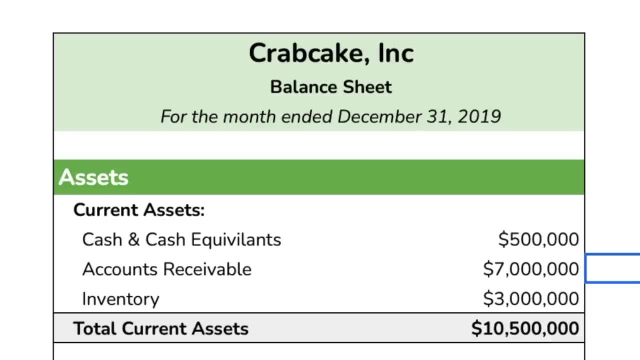 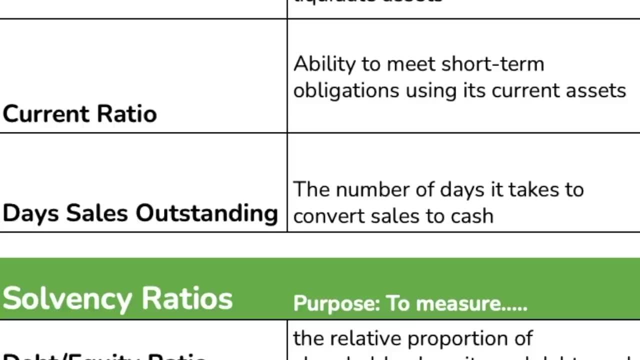 and then the second thing that the cfo will look at is the day sales outstanding. so basically, the sales outstanding is a financial statement or a balance sheet metric that will show us how far or how long it takes. so here we have day sales outstanding, which is the number of days. 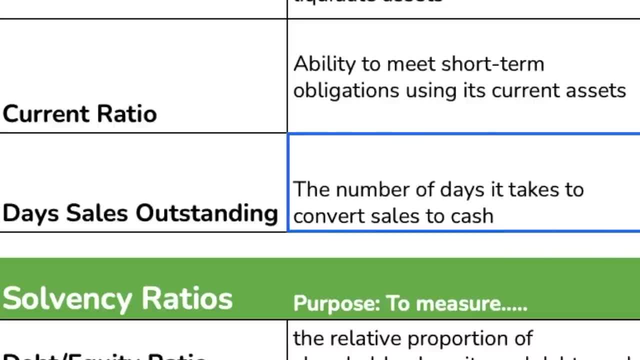 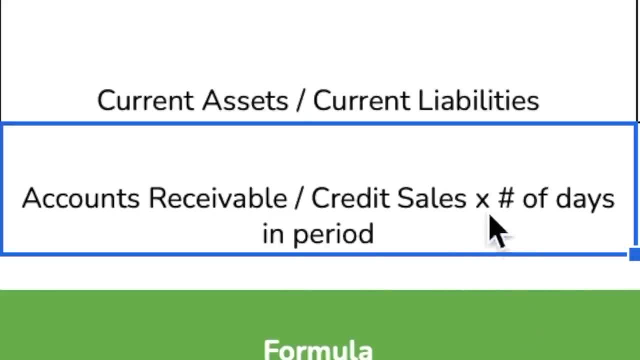 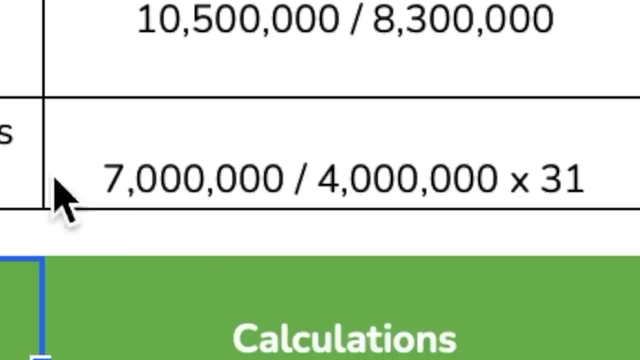 it takes to convert sales to cash, which basically takes the accounts receivable balance divided by credit sales and then multiply it by the number of days in the period. and to apply this to our example here, if we take um the accounts receivable balance, which is seven million dollars divided by 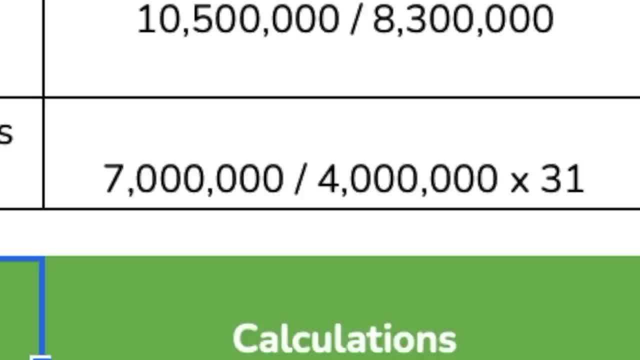 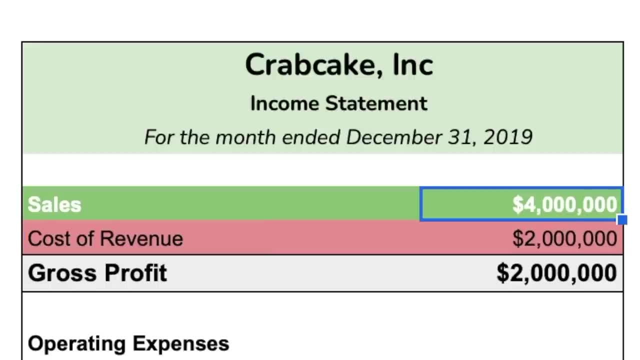 credit sales four million dollars, which we can see here in a balance sheet or the income statement. rather, if we switch over to the income statement, we have sales of four million dollars. so we take the number and we uh plug it here. so we have seven million ar divided by credit sales um four. 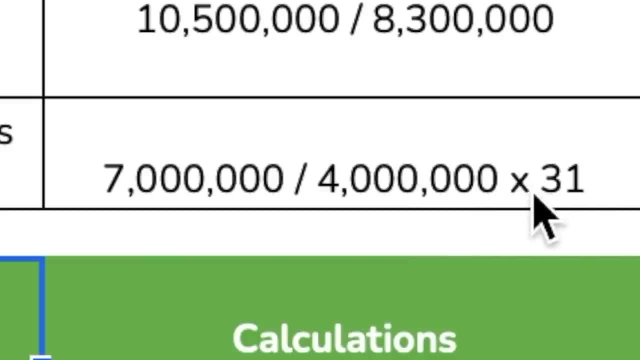 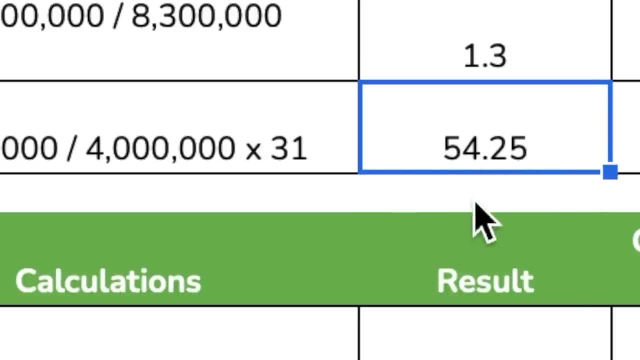 million dollars times 31 days. this happens to be a month with 31 days. um, then that gives us a result of 54 days. so 54 days. so this is saying that the company takes, on average, 54 days to convert its sales into cash. so this number is a little bit on. on the higher end, you want this number to always. 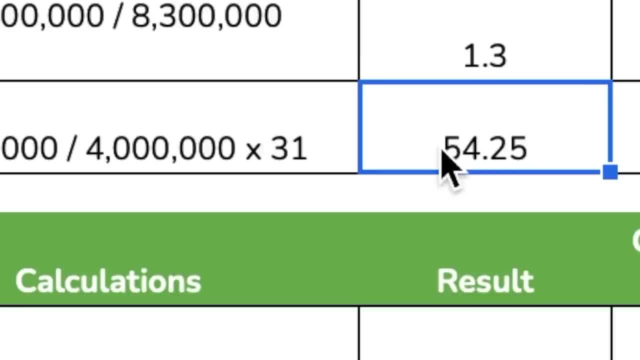 be somewhere around to 45 days. um, you know, if it goes up to 60 days, then it's a little bit above average. above 60 days, then that would be a bad signal. so these are the two things that the cfo would look at for. 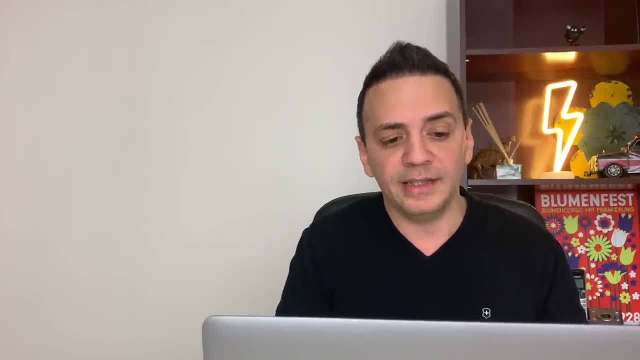 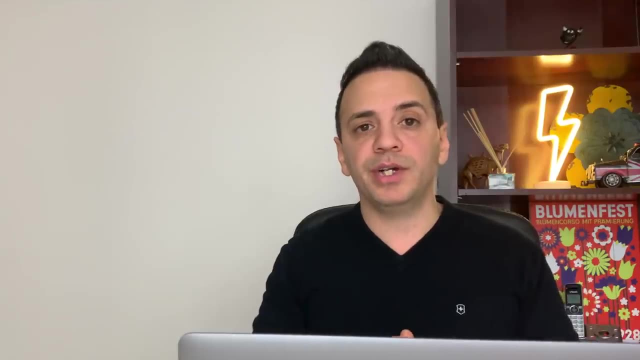 accounts receivable. uh, first is the aging schedule and then they will look at day sales outstanding or dso the next item in our list is inventory and basically when a cfo looks at inventory, they're looking at a balance of three million dollars in this case- and they want to make sure. 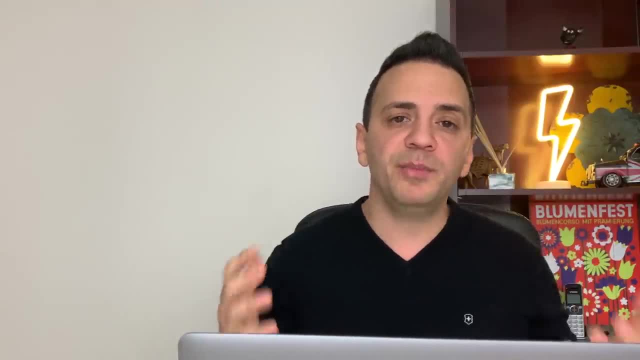 that none of it is nearing expiration or obsolescence. so if you have three million, three million dollars worth of inventory, it doesn't mean that all of it is sellable, right? maybe some of it is not. you're not, you're not going to be able to sell. so if you have 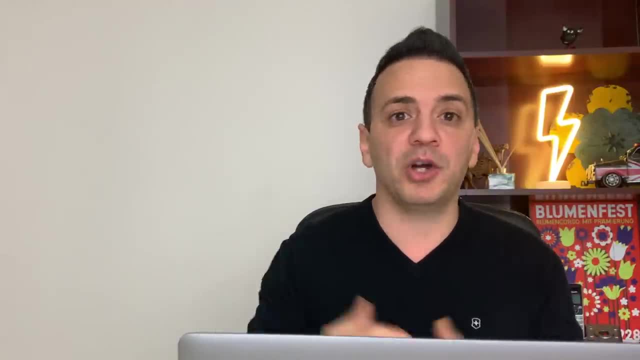 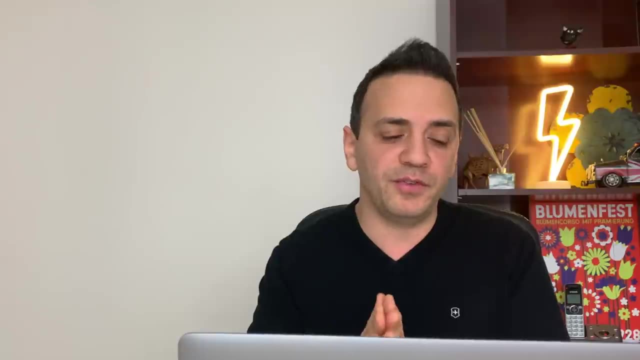 inventory, especially if it's like a food inventory and a big chunk of it is a food. products are nearing expiration or going to expire very soon, uh, so this is a risk here. so if you, if you're looking at an aging schedule of inventory, you can tell by bucket how much of this inventory 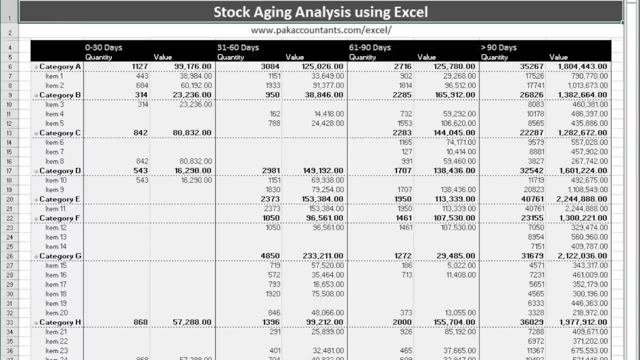 needs to be moved quickly in order not to be written off or not to lose money on it. so a cfo will look at a breakdown of what makes the three million dollars in this case to determine how much risk is associated with this inventory, how much of it needs to be moved quickly. so now we've covered. 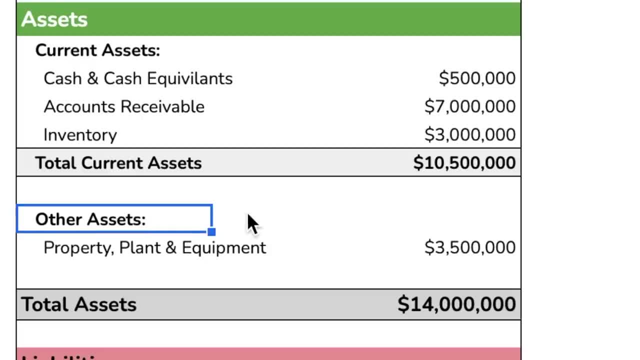 all of the items in current assets. so the next item here is non-current assets or other assets, and we have here property, plant and equipment. and when a cfo is looking at this balance of 3.5 million dollars, they're asking themselves a question of: is this entire balance appropriate? 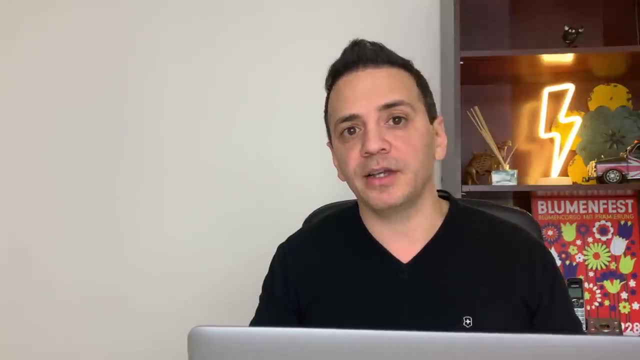 to be booked in a balance sheet, meaning, is any of this obsolete, like if this is machinery, or are we using all of it or some of it is obsolete and needs to be written off? so this is the risk here when you look at this number is to know the composition. look at a breakdown of the assets that 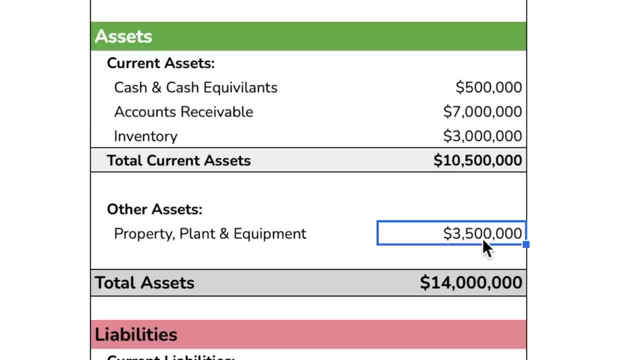 are included here and determine whether all of them are in use. all of them have a future economical life for the company? um. so this balance is appropriate. otherwise, if it's not, if a part of it needs to be written off, then that that's a hit to the p? l and that will reduce this number here. 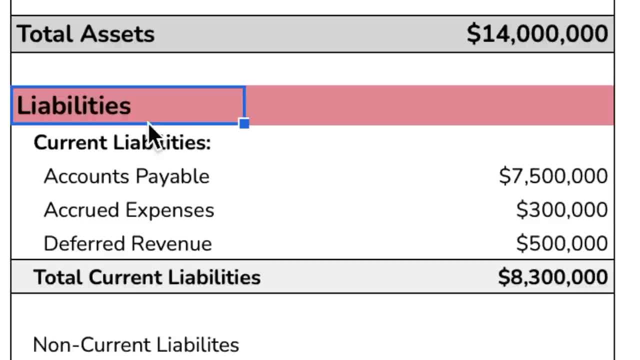 in the balance sheet, all right. so now that we've covered the cfo and the cfo, we're going to cover the assets. let's look at liabilities, and the first item in current liabilities is going to be accounts payable, and when a cfo looks at this number here, the balance 7.5 million dollars. 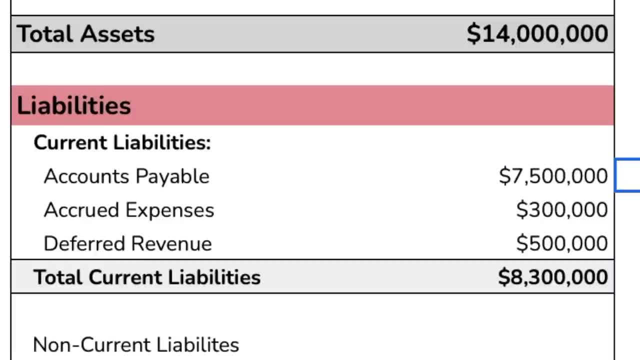 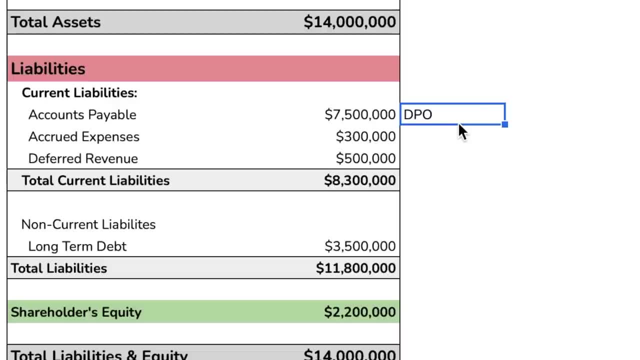 they think of two things in terms of risk when it comes to accounts payable. so the first thing: they think of dpo, or days payable outstanding, which is basically the amount of time that the company takes on average to pay- uh, to pay its obligations to vendors. so each company has a 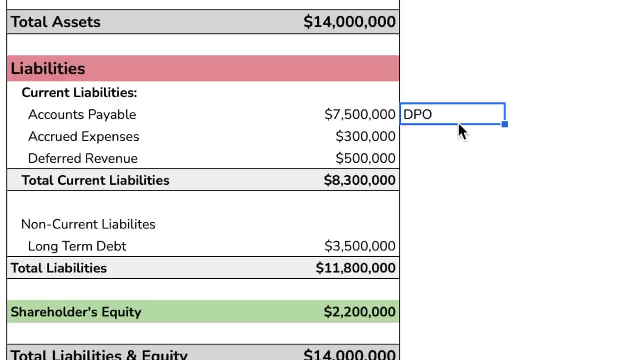 unique cycle of payment. sometimes it's a quick cycle of 30 days. uh, sometimes it's maybe 90 days, 120 days when it's a like a bigger supply chain, when you have vendors for your materials. so basically, the longer the better in this case, and the CFO be. 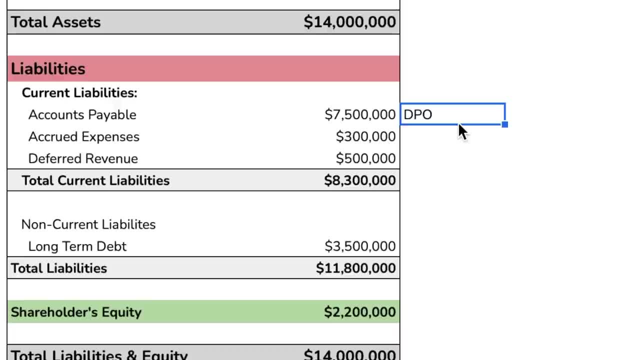 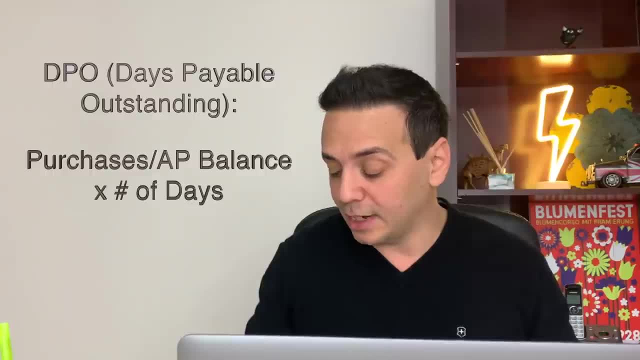 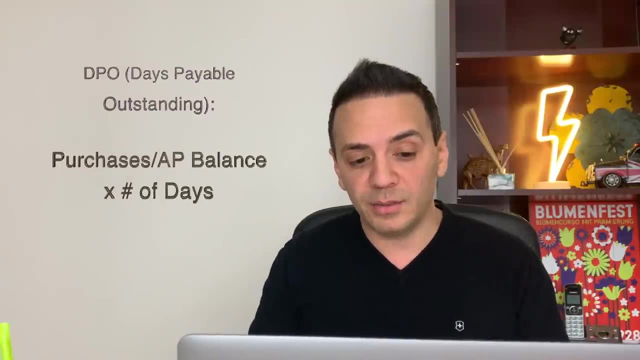 looking to measure the DPO and the DPO days payable outstanding. the formula for it is purchases on credit divided by the account accounts payable balance, and take that and multiply it by the number of days in the period and that would give you the DPO, and typically you want that number to be as long as possible. so 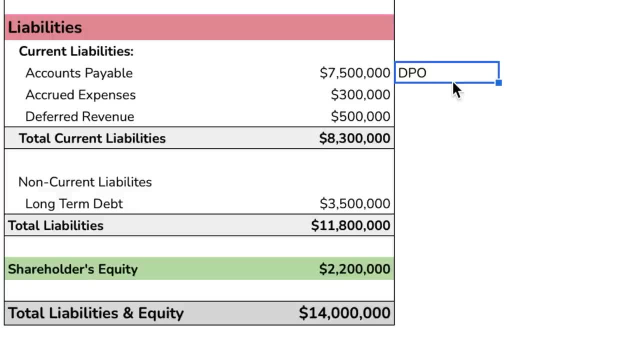 that you want to shrink your cycle of receiving from your customers and make the cycle as long as possible. so you have an advantage- and this is like a cash flow advantage- when you collect quickly and then pay off on the longer duration of time. so DPO is the first thing to look at and then the second. 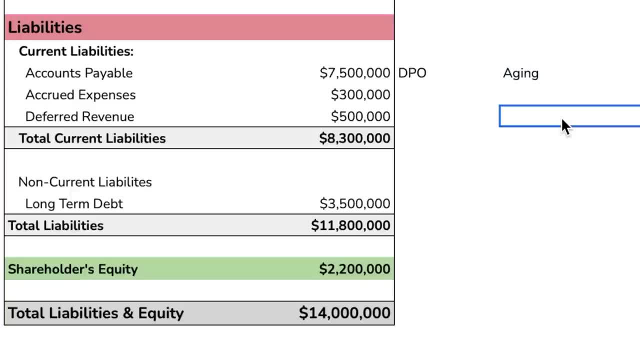 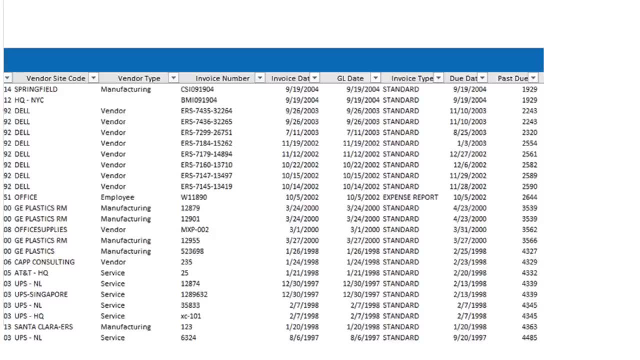 thing is gonna be aging. so you know, similar to when we talked about accounts receivable, when also, when we look at accounts payable, we want to look at the aging of the composition of the 7.5 million dollars to determine how, how much of it is current and how much of it is aged. 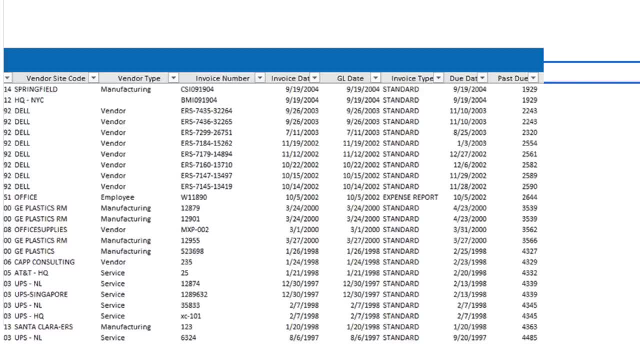 Because the risk here is that if a lot of this balance is aged, meaning that we owe this for the past- let's say maybe six months or so- this is a sign of trouble, right? So if the company has a lot of accounts payable, 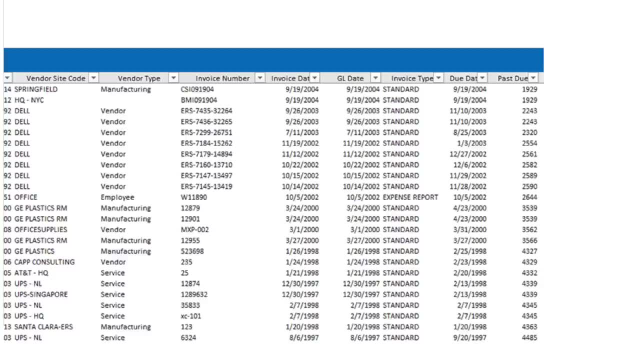 that is aged or that is past due. it means that the company isn't able to collect and time from its customers and pay off its vendors, So that's why it's really important to look at aging. That would give you a quick idea. 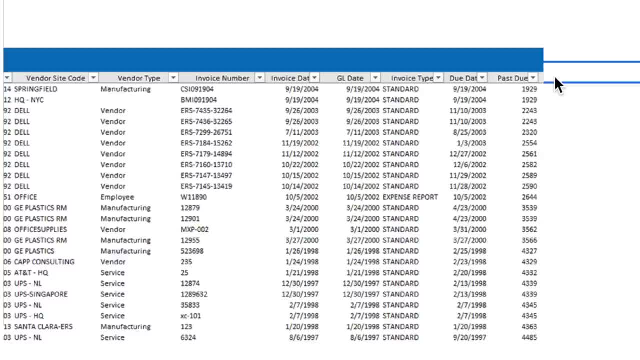 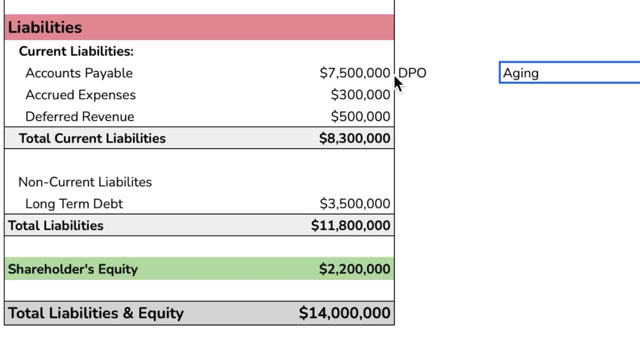 Obviously, when you look at the aging schedule, you want as much as possible of that $7.5 million to be sitting in the current section of the aging schedule and not being past due. So this is what the CFO would look at when it comes to accounts payable. 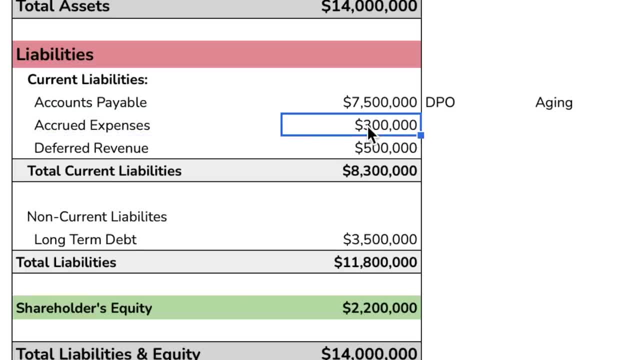 The next item is gonna be accrued expenses, and we have $300,000. And we said before- the accrued expenses is what the company's accruing for in terms of liabilities- that the company haven't received an invoice from a vendor yet. So what the CFO would look at here is: 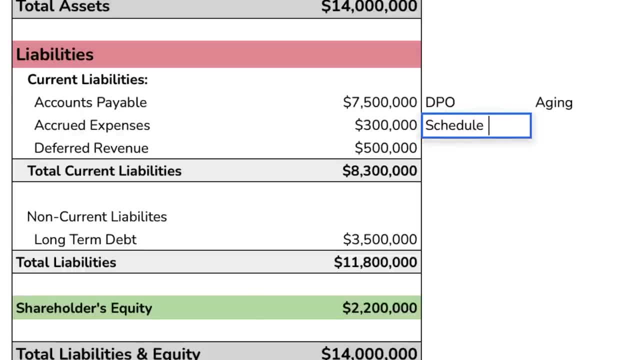 he would ask for a schedule. He would look at the number of this number here just to determine whether the company is appropriately accruing for everything that it owes. So only when you see a breakdown of the number, that's when you can make that determination. 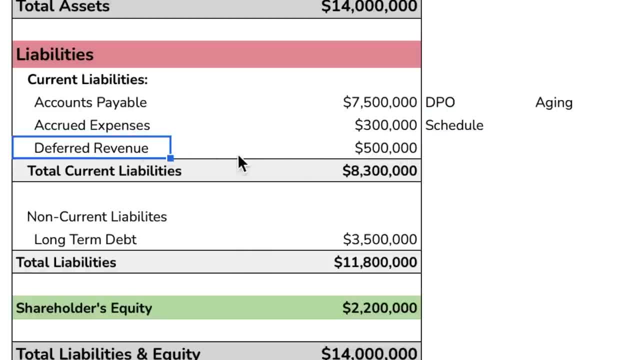 So a schedule here would give you an idea. And then the next item is gonna be deferred revenue. So a CFO would look at this number and think, okay, this $500,000 is received in advance from customers for future services or products. 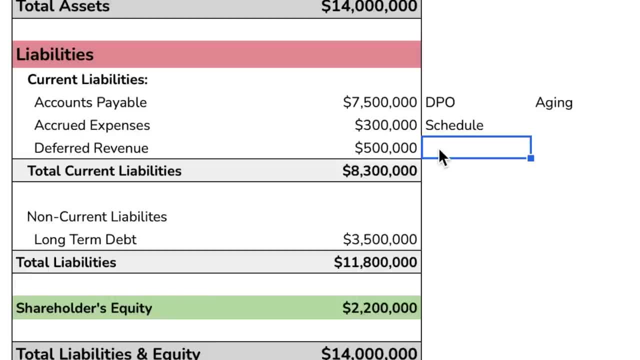 So he is actually going to be able to make good on this obligation. So the CFO would wanna look at and see what the customer is paying for. Let's say he's paying for a product and then will ask a question: okay, this is a product that we have on hand. 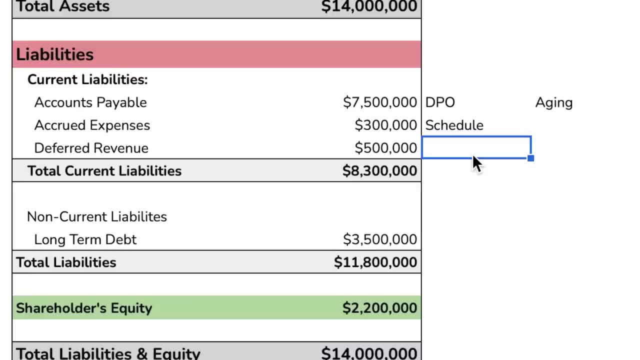 Is this something that we need to manufacture from scratch? Are we gonna be able to make good on this obligation here, And so you need to know what's included in this number. here And again, this is usually gonna be a schedule that you can obtain. 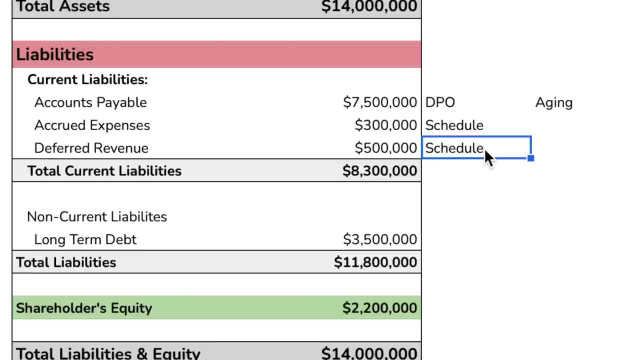 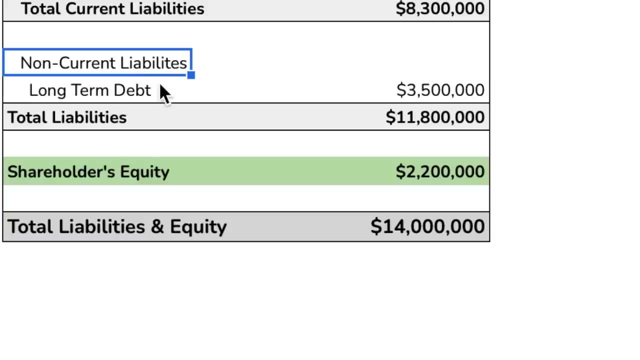 that the company needs to make good on. it should keep a schedule of all of the prepayments that it receives from customers. So this covers pretty much the section current liabilities. Now we come to non-current liabilities, and the CFO will look here and see that the company has a long-term debt of 3.5 million. And so the first 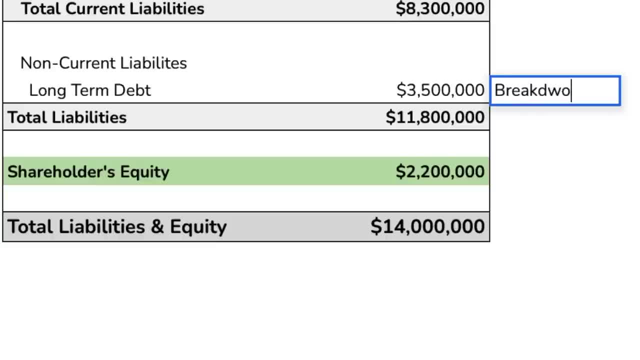 question is to ask for a breakdown of this number to see, just to see, the maturity, right. So you want to see the breakdown by maturity date of you know when do we expect to pay off this number? Is this made up of loans that are like three-year or five-year or 10-year loan? So basically then, 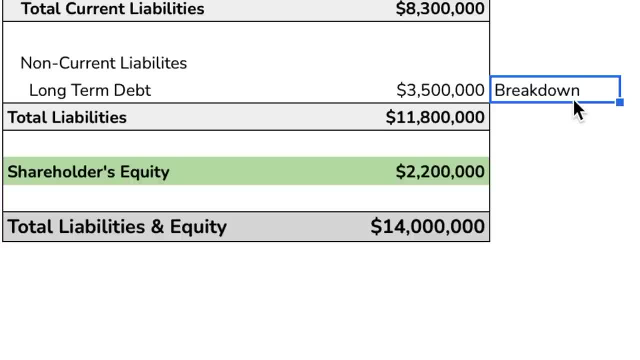 you can plan in the future. you know how you're going to pay off this loan. It's similar to when you own a house or a property and you want to know how long is the mortgage right? Is it a 10-year? 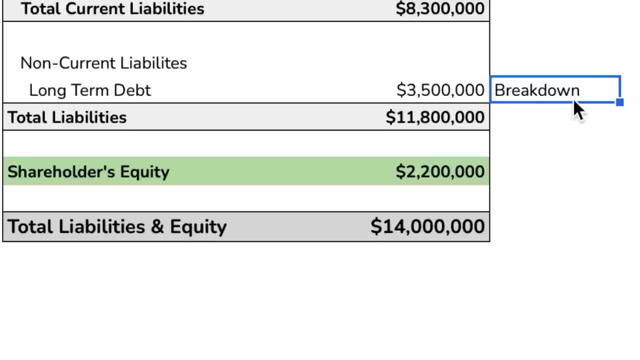 20-year, 30-year mortgage. It's the same thing here. If you have a long-term debt, first thing you want to know is how long will it take to pay off or what is the maturity date of this loan. So you come to total liabilities and it's $11.8 million And there are a couple of 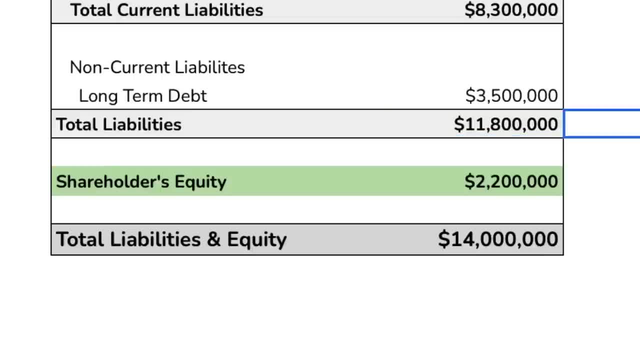 financial metrics, or KPIs, that you want to be using here to make sure that the company financial health is not something that is in jeopardy. So the first thing you want to compare is total liabilities. You want to compare that to equity And this is a financial metric here. 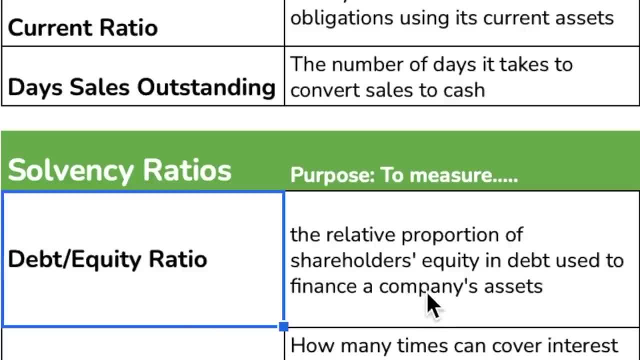 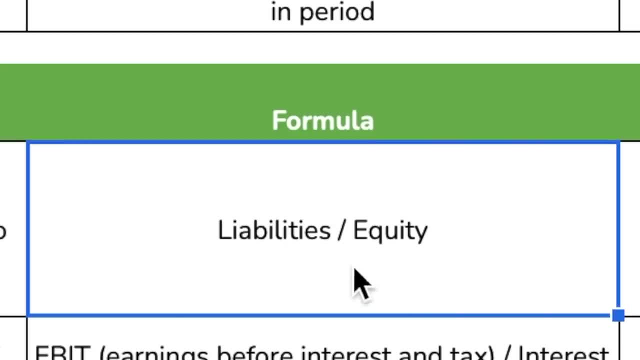 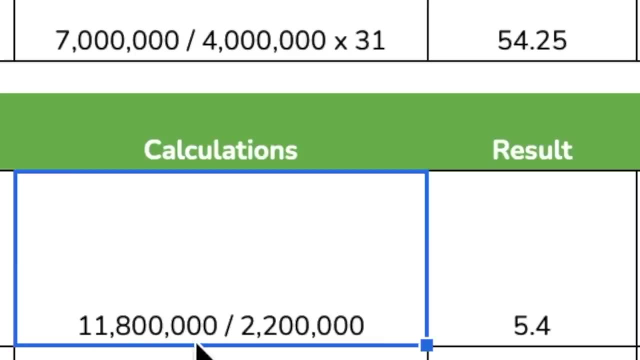 that is called a debt to equity ratio, which is the relative proportion of shareholders' equity in debt used in financing the company's assets. So the formula for it is liabilities divided by equity, And if we apply this here, liabilities is $11.8 million divided by equity, which is $2.2 million, And it will give us a. 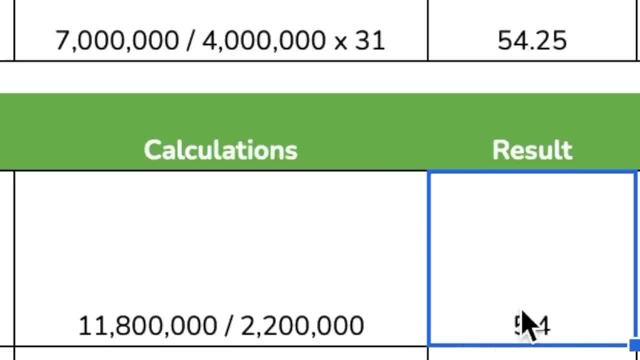 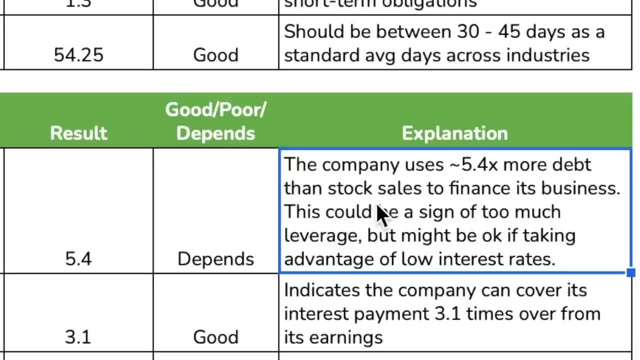 result here, that is 5.4.. So this number 5.4 is saying that the company is using 5.4 times more debt than stock to finance its business. This could be a sign of too much leverage, but it might be also the company taking advantage of low interest rates. So there are two sources of 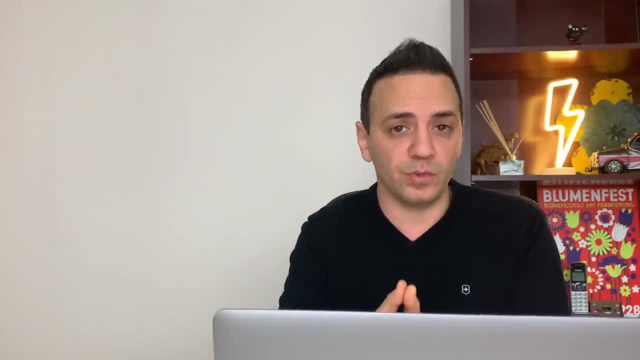 financing for the company. It's either raising debt, in this case, which is the long-term debt, or selling stock, which is equity, And so each one of them has a cost to the company, and it's up to the company to determine which one is cheaper. 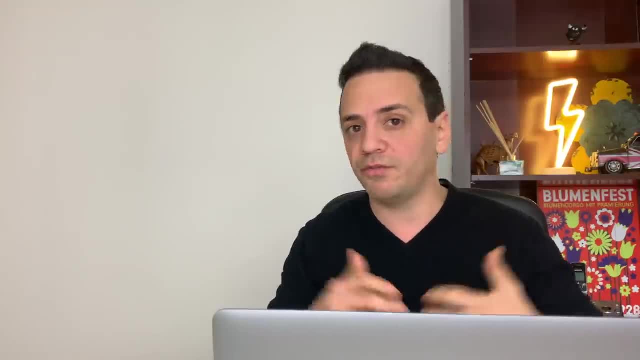 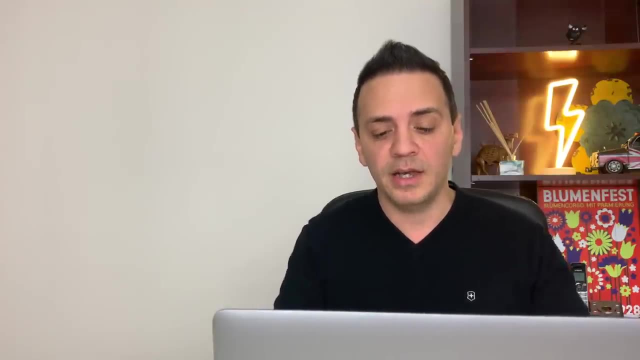 If the interest rates are low, in an environment where the Feds are lowering the interest rate, then it makes sense for the company to raise more money from debt over financing. And so in this case, here you look at this metric and you can determine the debt to equity ratio. The other 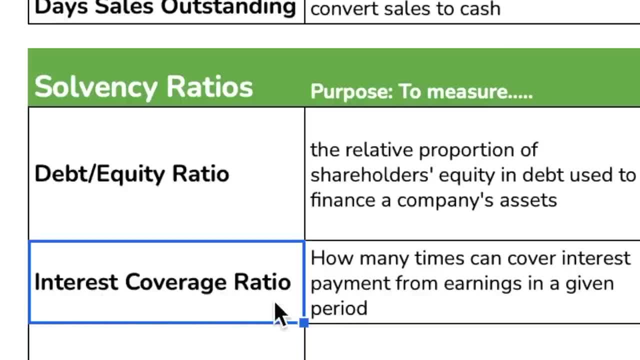 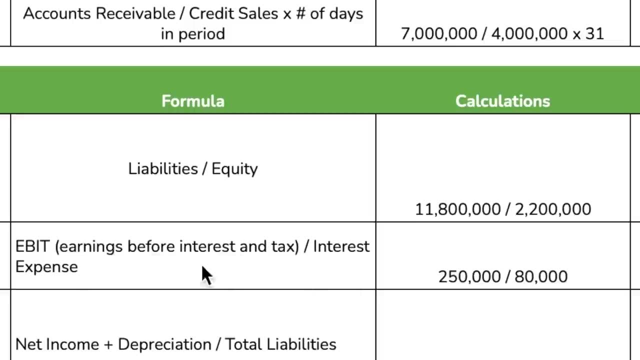 financial metric to look at here is a loan rate, and this number shows the loan rate to equity ratio and the financing of the loan itself, which is the interest coverage ratio. So this is measuring how many times can a company cover the interest payment from earnings in a given period, And so basically take the earnings, or EBIT, in. 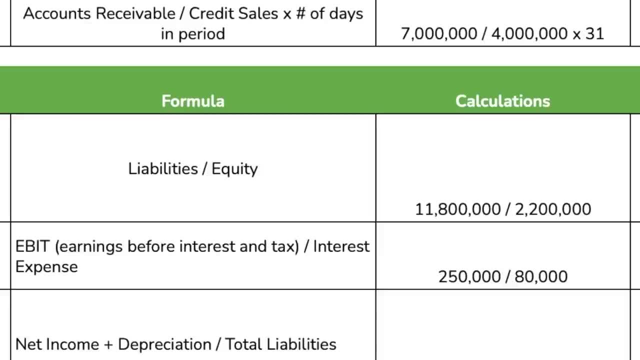 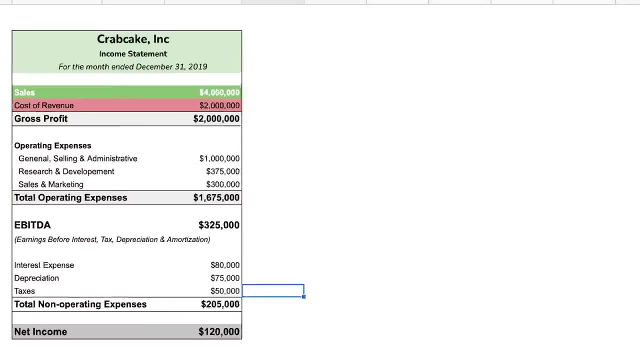 this case earning before interest and tax, divided by the interest expense. And so in this case it's 250,000, which we can get here from the income statement When you take the EBIT, which is earnings before interest and tax, 250,000 divided by 80,000, which is the interest ratio, the interest rate and the 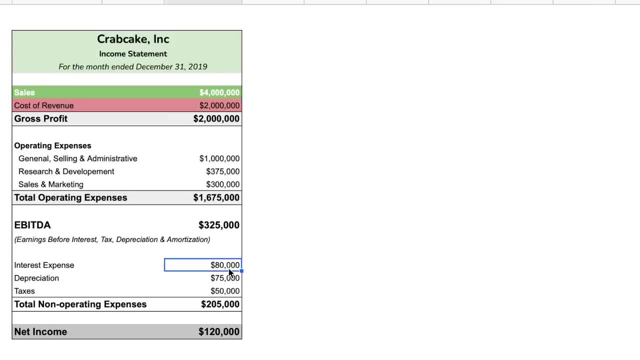 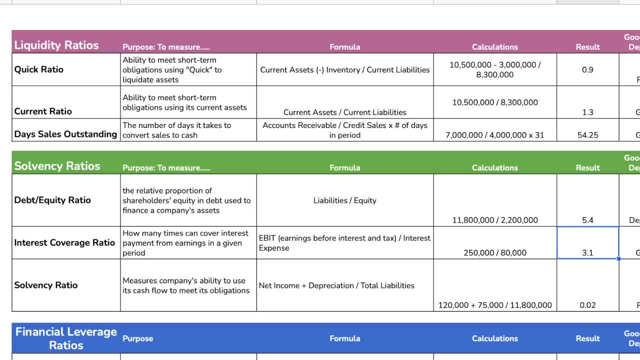 expense. again, that's from the income statement here as well- $80,000 of interest expense and the result is 3.1. and so this is saying that the company can cover its interest payment three times, or three point one times, over its earnings, and so this is good. so the company has makes enough in earnings to 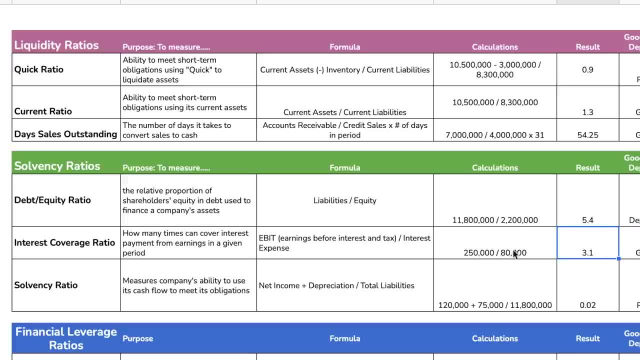 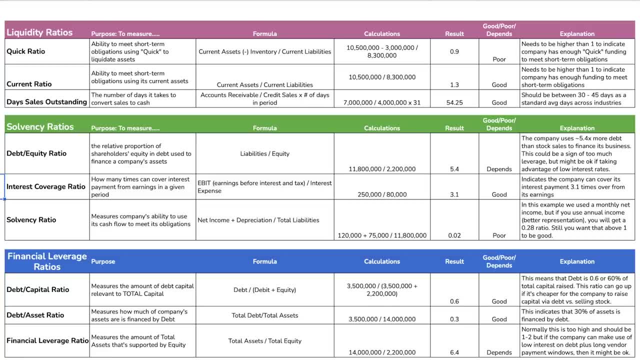 cover its interest by a factor of three, so this is a good sign that the company is in fact is able to service its interest on the actual loan. there are a few other important ratios, such as the liquidity ratios- quick and current ratios- that are used by CFOs to analyze the balance sheet, and also there are 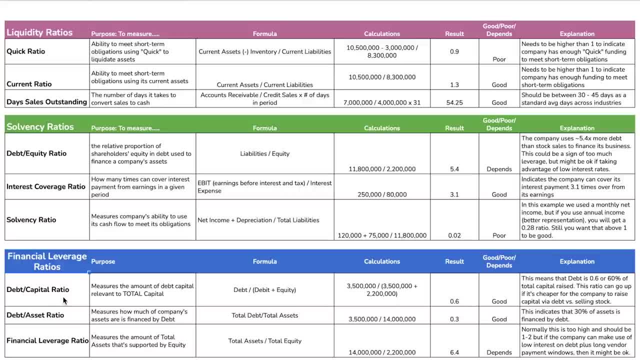 financial leverage ratios, such as the debt to capital ratio and debt to asset ratio, as well as the financial leverage ratio, and these are all are important ratios that the CFOs use to analyze a company. I'm gonna leave a link to this file down below you description in Excel so you can download it and look at the balance sheet. the. 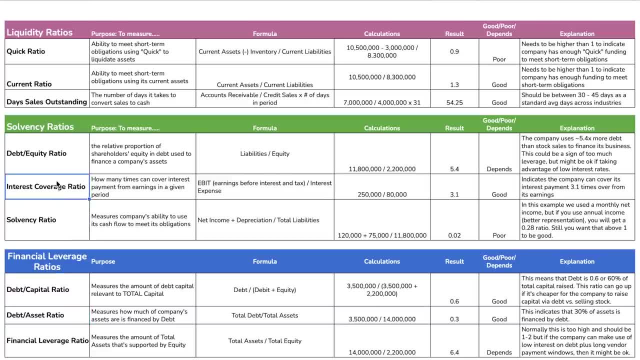 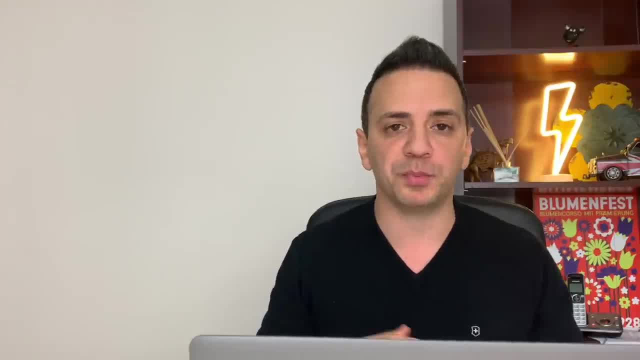 income statement and the actual ratios that are used here. so you can find a description. you can find a link in the description down below. so the link in the description below will lead you to a product on my website to purchase, which is really inexpensive and it includes the Excel file that we discussed today. 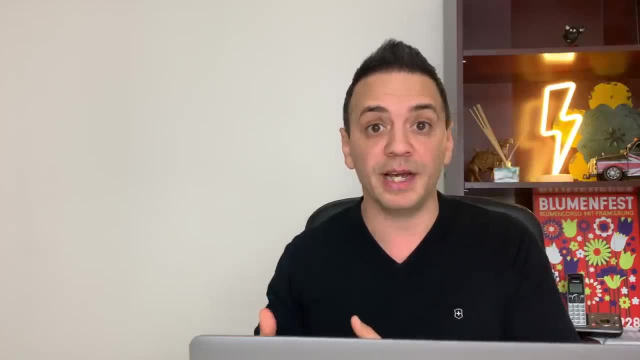 with its balance sheet, income statement and financial metrics formula and interpretation, and also an actual PDF summary, a one-page summary of the of the metrics that we looked at today. so you can you can keep it as a handy reference for the future. the reason why this is a paid: 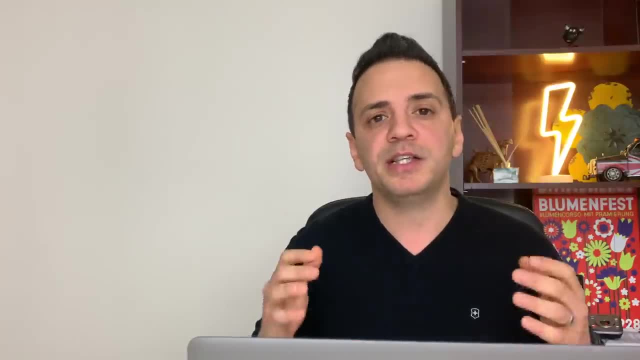 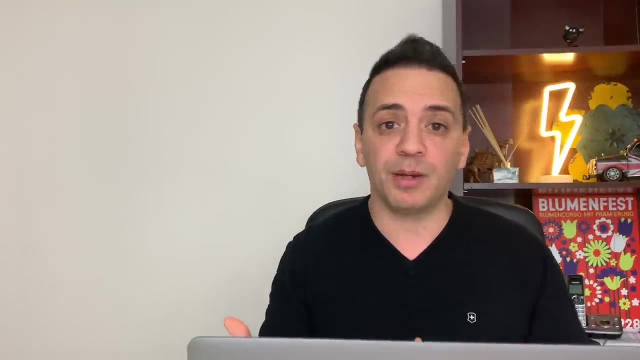 product versus a free giveaway which sometimes I give on this channel, is because this, this template, took a lot of time for me to put together and test and make sure that it's correct and accurate, and also because when you buy a product through this channel, you're also supporting the channel, making sure that. 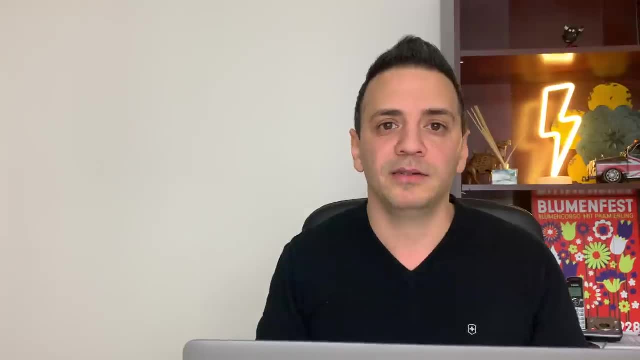 I'm able to give you the content, or the free content, that I put out every week. that's it for this video. if you liked it and you learned something new from it, give it a big, fat thumbs up and share this video with someone that you think might benefit from it, and I'll see you next time.